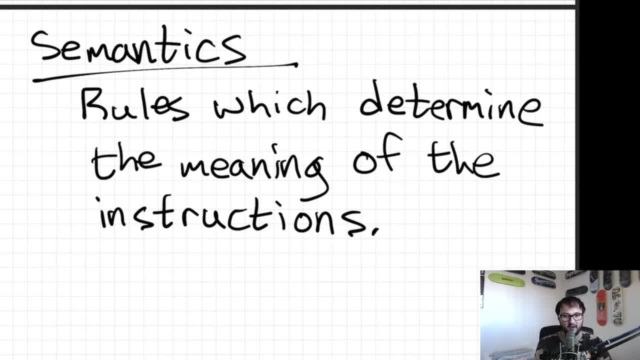 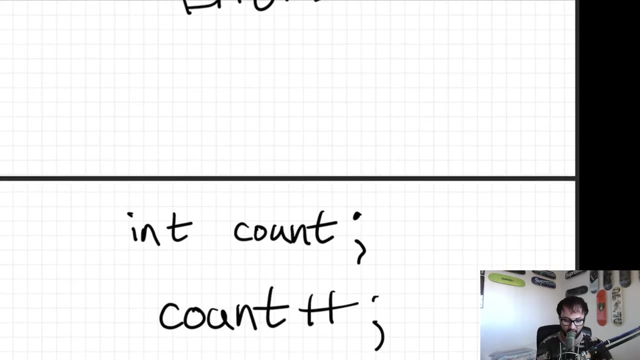 five into a variable. I'm calling x. I want to count all the apples in the orchard. I want to count all the Macs at the store. I want to. there's so many examples of semantics. there's endless ones, And those are going to be run time errors, So something like: 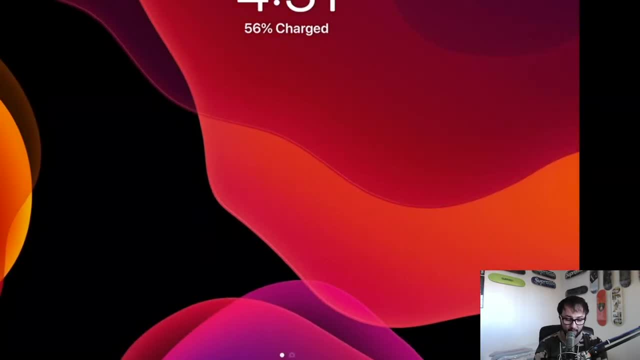 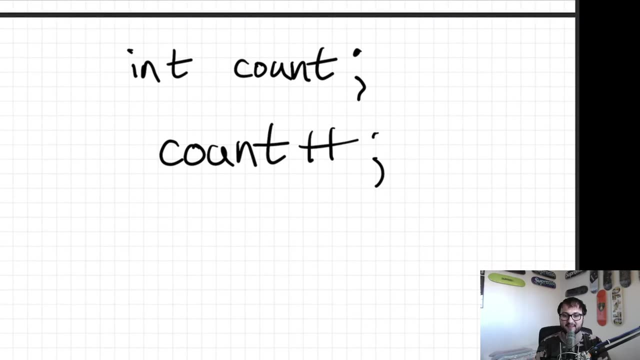 your program compiles completely fine. turned off my iPad there- Completely fine, Except for when it's running. you're getting all these errors and it's just. you have no, no clue why your program is spitting out the output that it is. 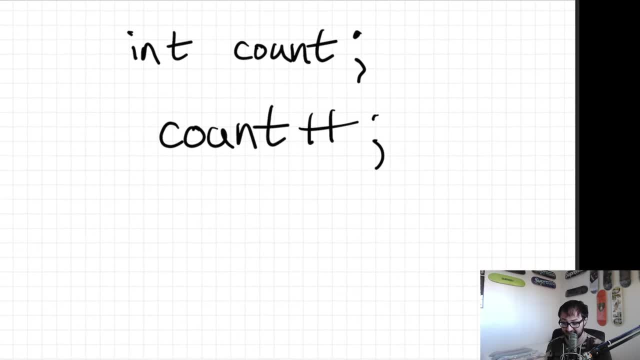 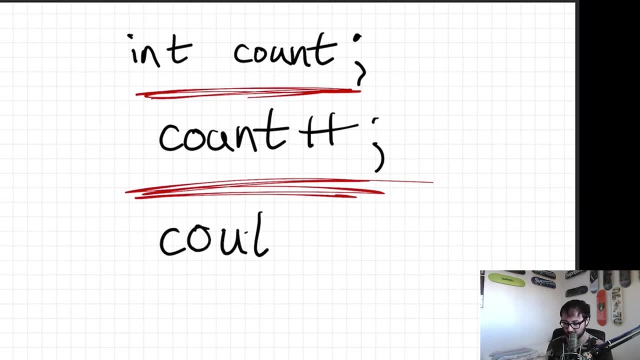 Such as in the classic count example where you forget to initialize your variables. you increment your count and then say: come down and see out your count. You're going to get, say this got 65 in it. you're going to increment that to 66, expecting: 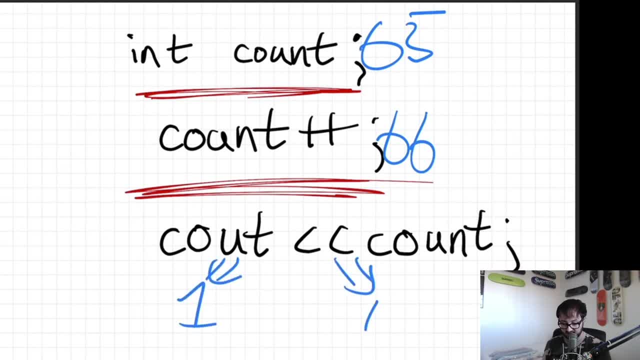 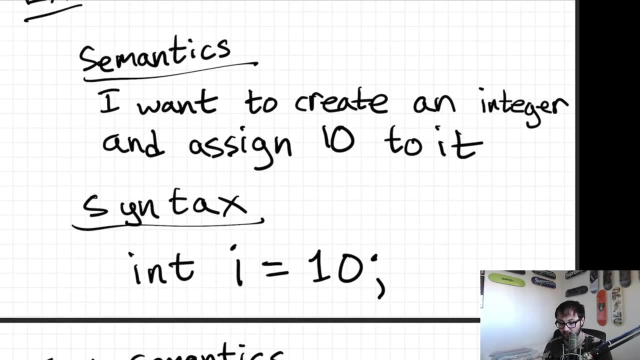 one to come out, but you're really going to get 66 to come out. That is an example of a semantics error, And there's so many more semantics errors that you can run into. That's just one of the one of the so many possibilities. 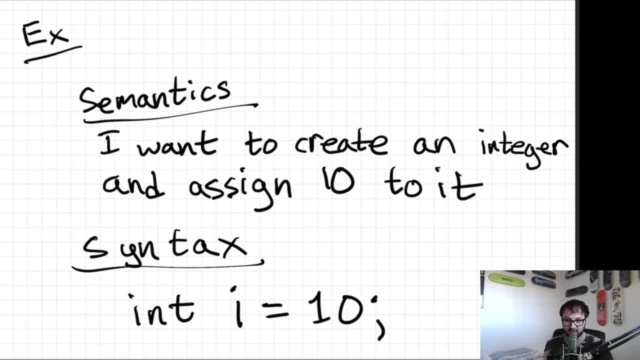 So here's a couple of examples of syntax versus semantics. So in this one I want to create an integer and assign 10 to it. So here I'm creating an integer. I want to create an integer and assign 10 to it, and assign 10 to it. 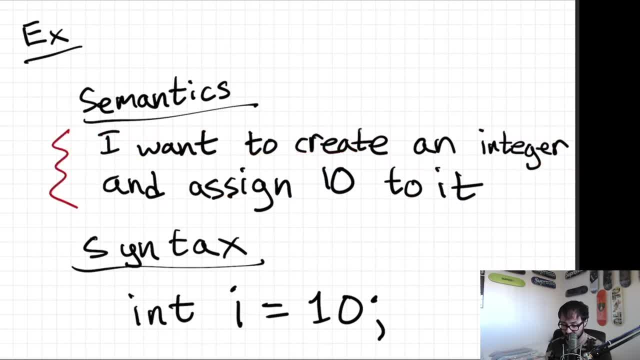 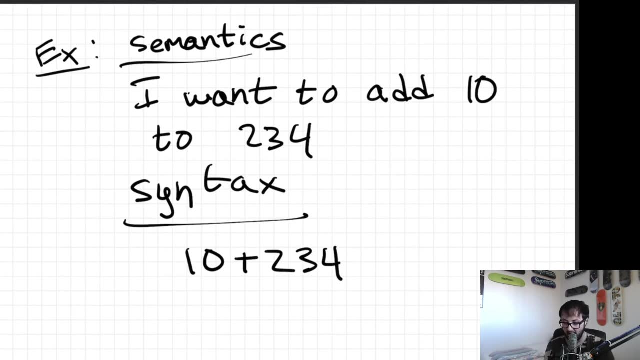 So this is going to be your semantics, This is going to be your syntax. This is what you're thinking in your head. This is what the computer can read. One more example of that is going to be: I want to add 10 to 230. 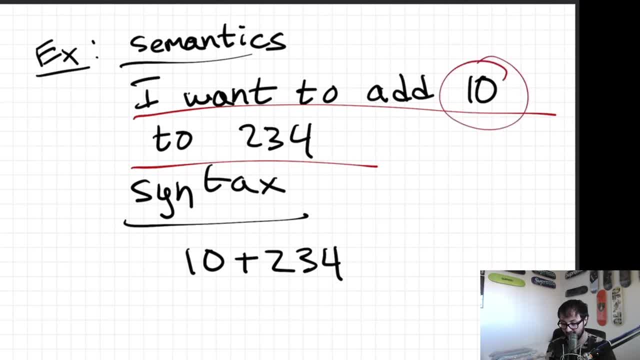 Okay, 234.. So I want to take 10 and 234 and I want to add them together And this is something that your computer can read. This is something your computer can read And this is something that you think up in your head that a computer cannot read.